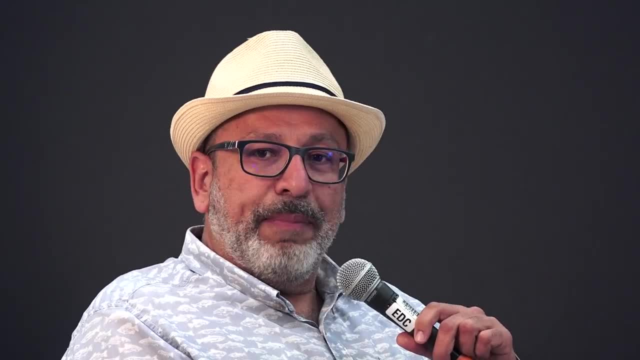 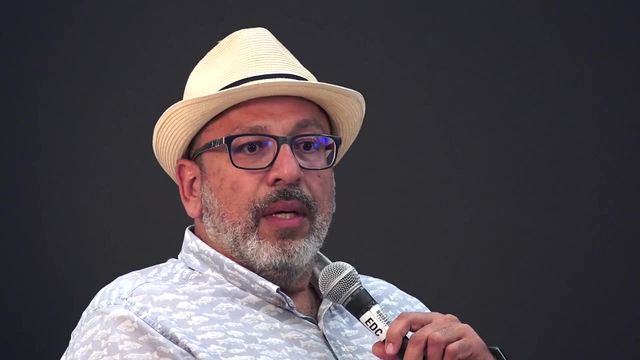 over the years we've been able to see the patterns of illness we see in nature. And over the years- that 400 years- these early microbiologists began looking at not only those sort of first glimpses into the microbial world but really relating it to the chemistry and the physical. 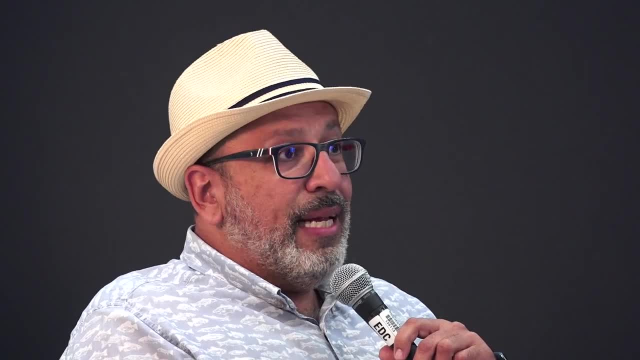 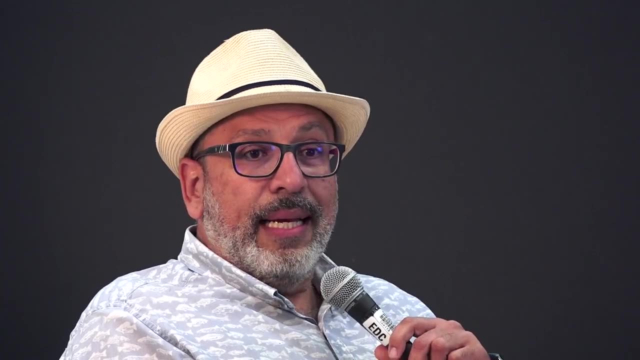 conditions, the hydrology, the human migration and distribution. all of it to really understand what these organisms were doing. And as EEB continued to grow- or rather environmental biology, I should say, continued to mature, we began to see scientists. 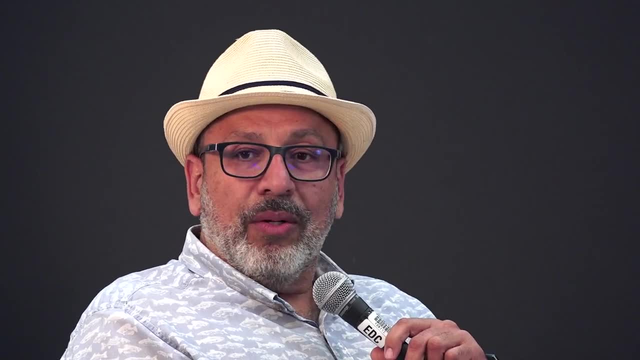 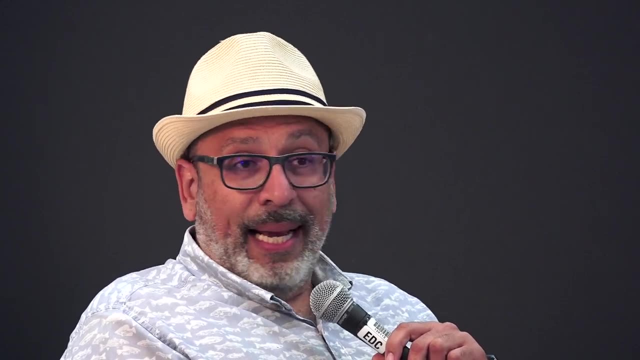 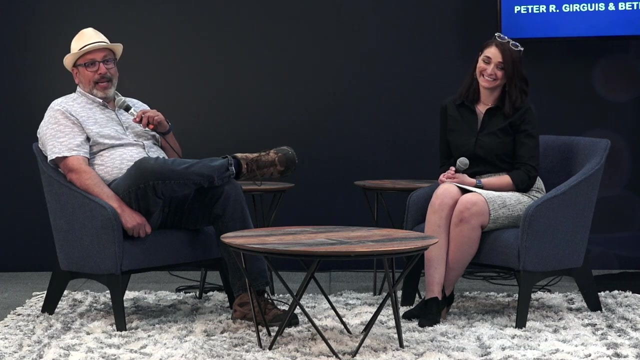 looking at how microbes shape the chemical environment around us. Right, And we know that microbes- I mean today- we know that they're the stewards of our planet. right, They run the biosphere. I believe that we humans are incidental, So if you wiped out all of us, the planet would. go on Many ways. better right, But if you wiped out all the microbes, we would no longer have a biosphere. It would come to a halt. This community of environmental microbiologists has been really thinking about how we can shape the chemical environment around us, And we've been able to. 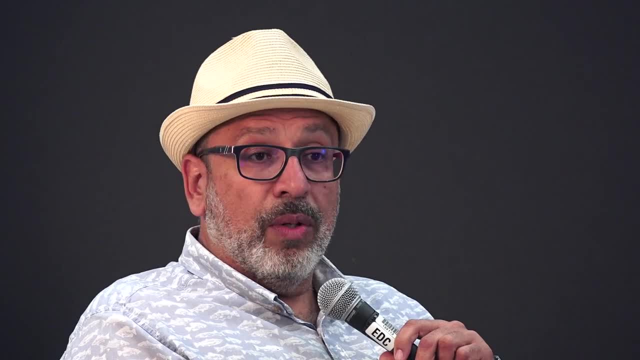 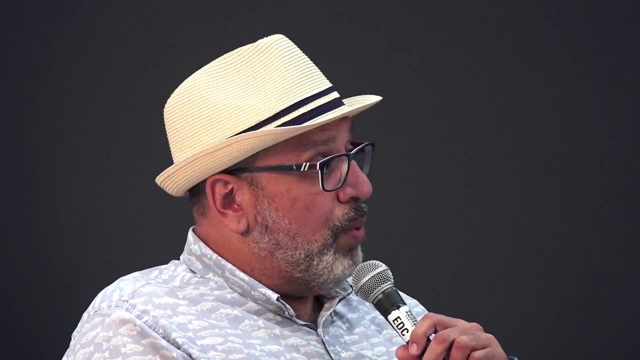 think long and hard about the relationships between microbes and the world around us- chemistry, hydrology, you name it- And in many ways EEB has played this really special role in ASM of thinking about the relationships between microbes and other planetary processes And 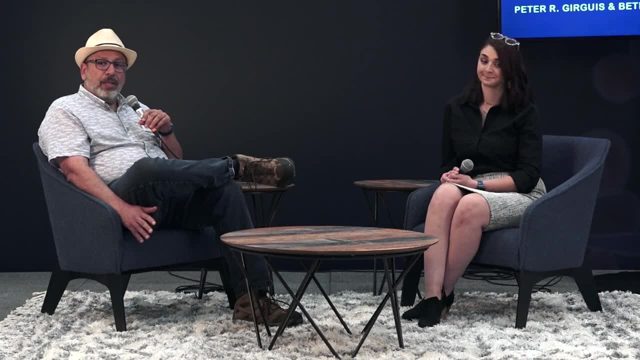 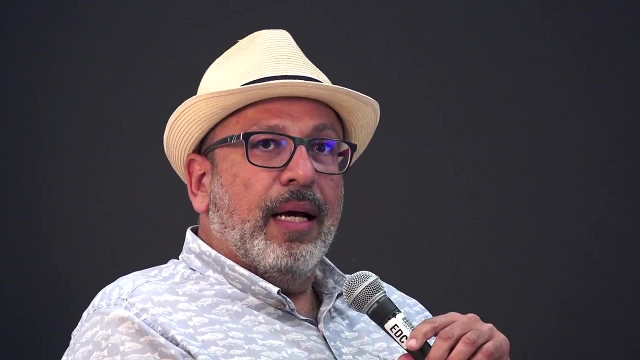 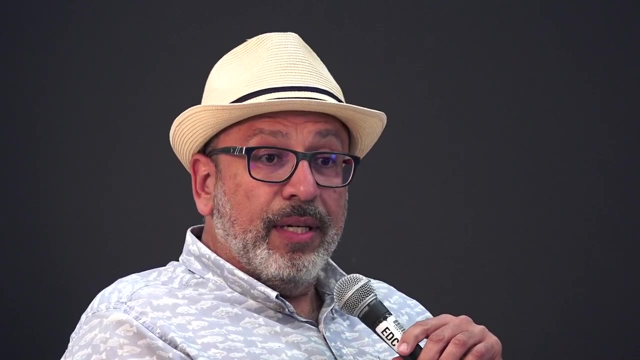 frankly, other anthropocentric processes. Why do some human populations get sick and others don't? Today we find ourselves on the cusp of trying to use our more contemporary technologies to answer many of these same questions. right, We've learned a lot in 400 years. 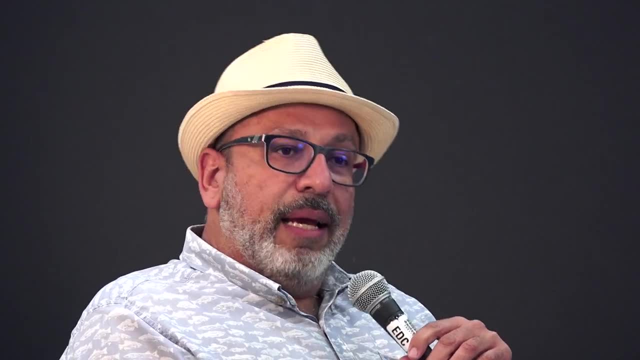 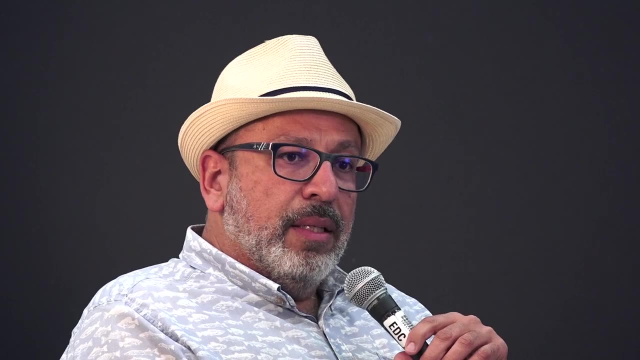 but we have so, so much to learn, And today we've been. we wanted to talk with you a bit about what the EEB community has been doing and then, of course, where we're headed. So one of the things, Beth, I was really keen on talking with you about here was, you know from your point of view. 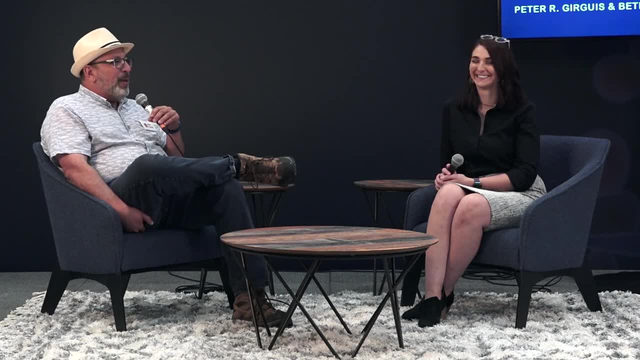 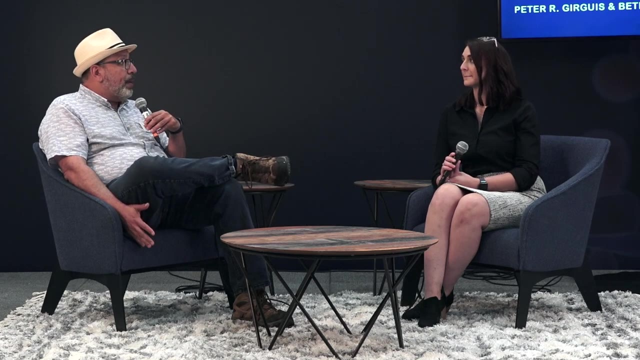 with your ASM hat on, as they say, and having been a part of this EEB retreat, what are some of the ways in which you think EEB can play a role, not only in working with ASM to advance EEB, but to really help our community better relate? microbiological data. 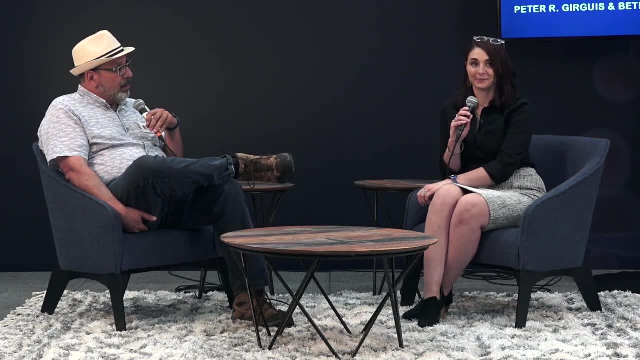 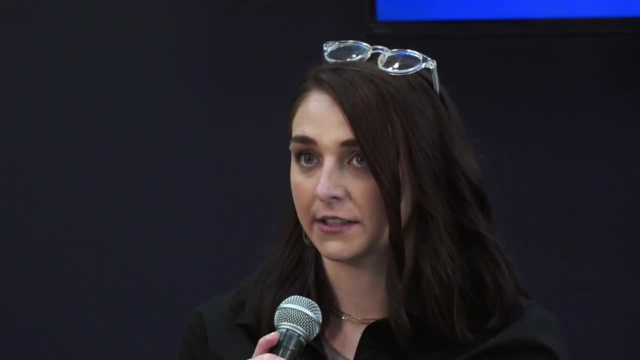 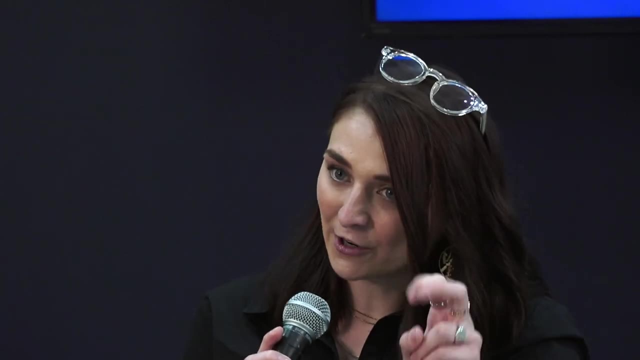 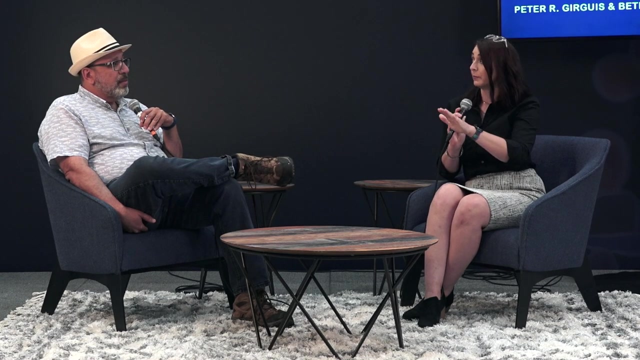 It still goes back to the small aspect And you take a look across the microbiology field and, although the data might be written in a different language per se, it's still part of what it means to be a part of microbiology, just on that level. 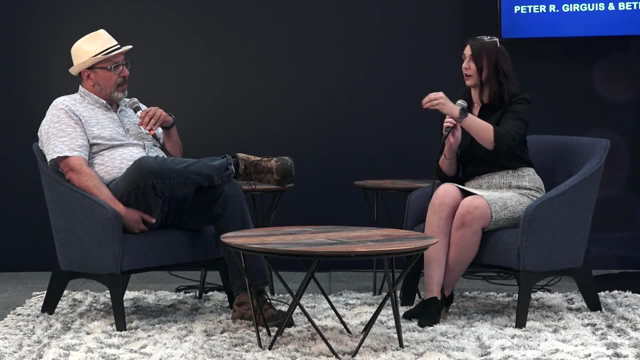 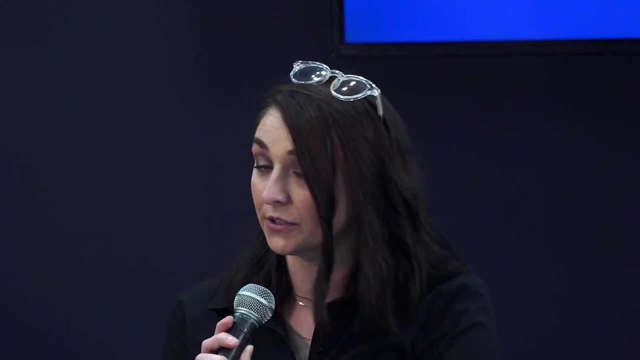 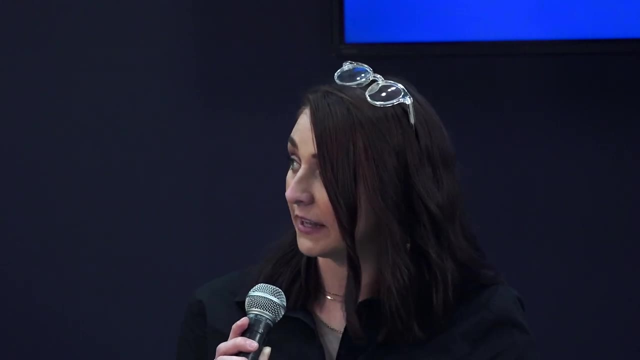 And then you're looking at how can we then create these cross communities across EEB, across with host microbe, because there is both a lot of nuances but there's also a lot of broad big areas of where the science is really going and ASM's place, of how best to help support the science for those. 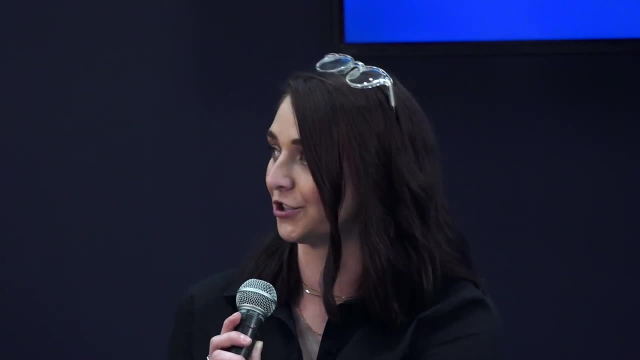 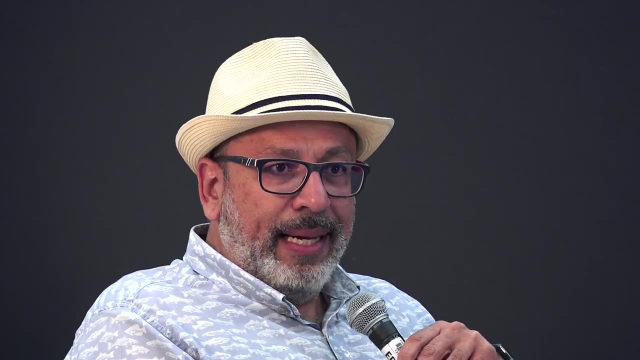 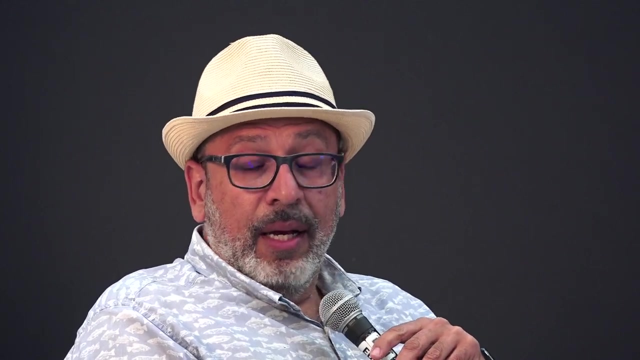 directions, both the nuance as well as the big, big picture. Yeah, that's a really great way of summing it up, because, as we were working together on this retreat to think about where is the EEB community headed, we realized that this is a community that has a deep understanding of how. 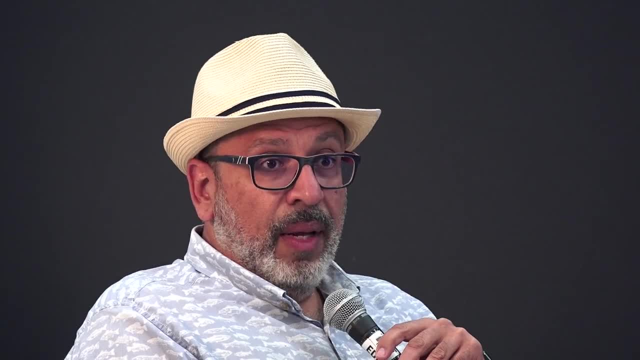 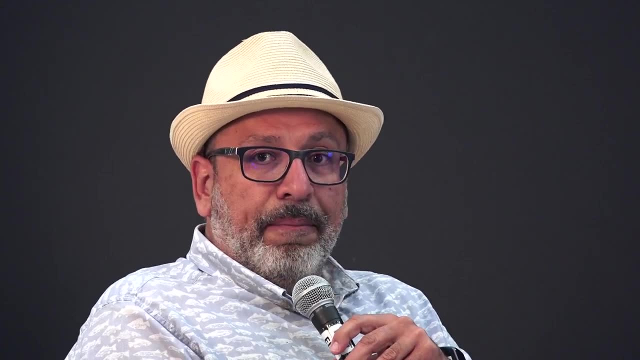 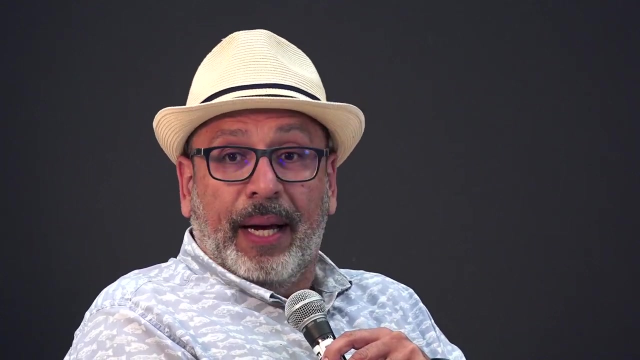 to deal with big and complex data sets, And we've been doing this for a long time And it occurred to us that there's a lot of value in offering that perspective to other communities for whom this might be newer. Perhaps the human gut microbiome community might be a good example. 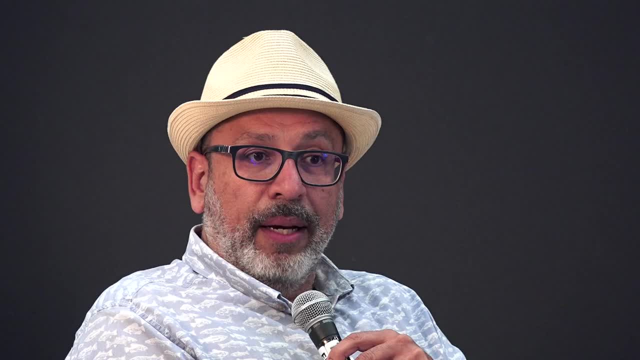 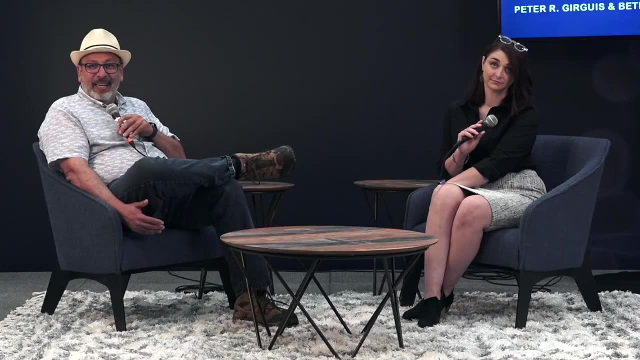 As many colleagues of mine at my institution study human gut microbiomes, as many colleagues of mine at my institution study human gut microbiomes, they turn to myself and my colleagues and say: how do you make a chemical measurement at an appropriate scale? How do you understand the fate of compounds as they advect or diffuse? 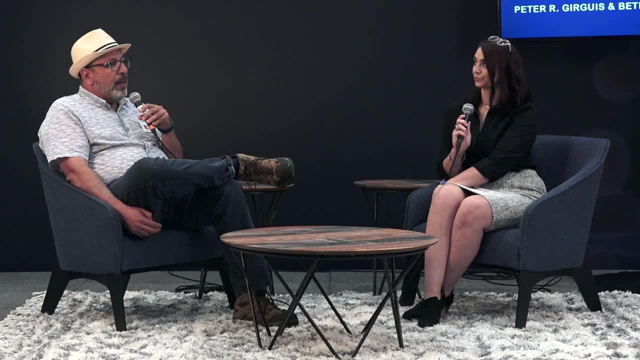 through an environment. And so I think, Beth, that what I'm inspired by hearing you say and others in ASM governance, is that you all will work with this EEB community to kind of provide the opportunities for us to engage with other communities, Absolutely, And so one of the things 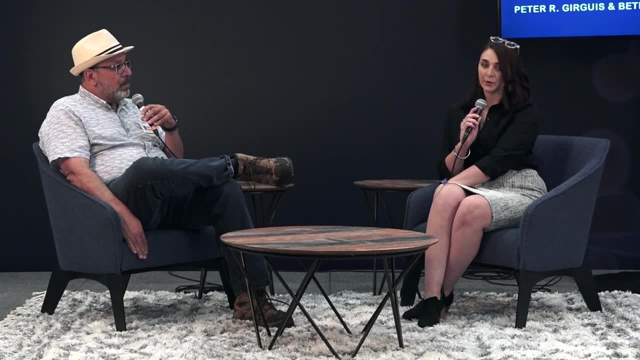 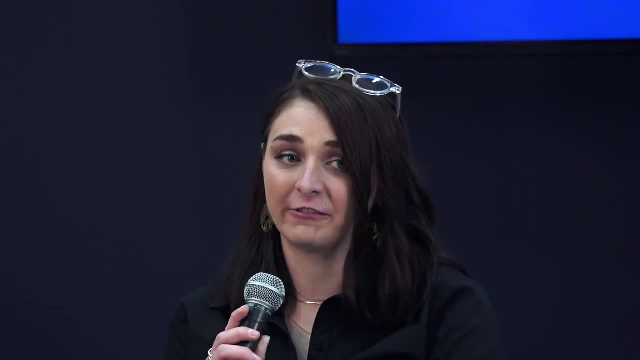 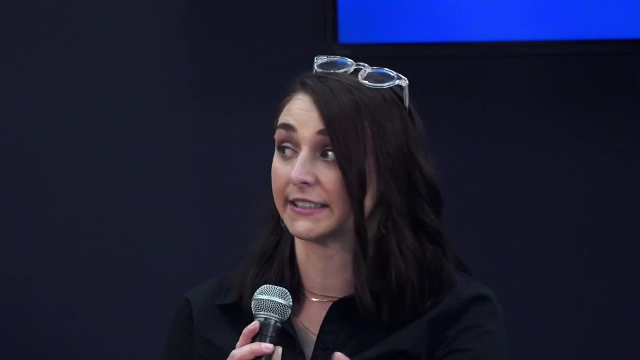 with antimicrobial agents and resistance. I think one of the things that we also have to consider with that. like they have their own booth, they have their own talks, but all of that relates back to ecology, back to evolution. You're not going to get resistance in a microbe unless it sees. 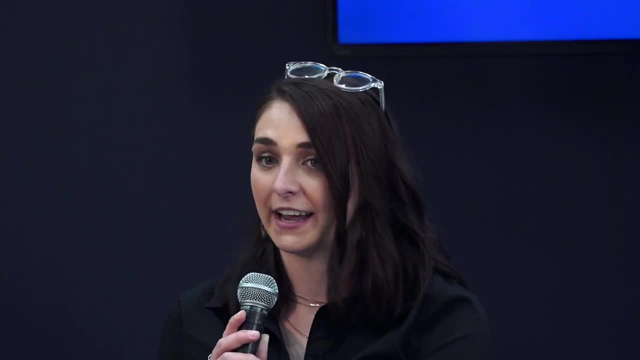 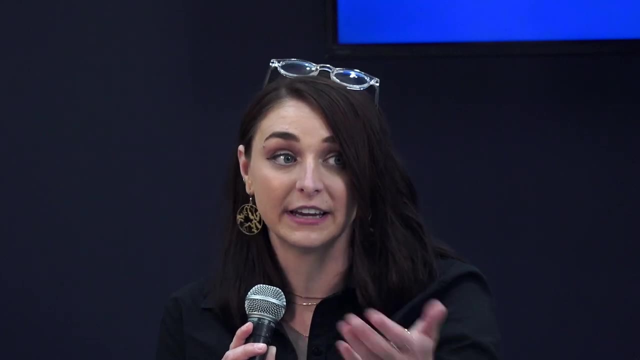 something to become resistant to. You're not going to have them, and that's where are they like. you have the genetic evolution aspect, but you also have the ecology. They're in an environment that can see it. So how can we then work like that is already naturally crossing just two? 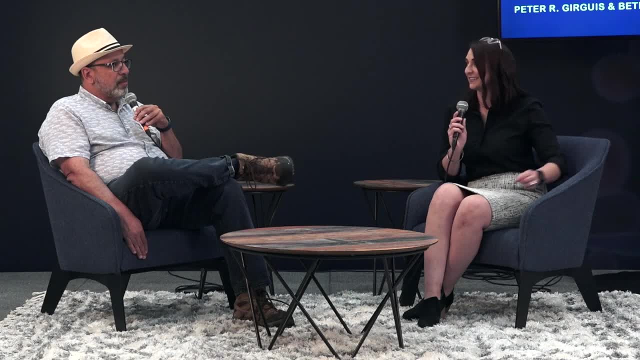 and then you take that further and then you bring in the human aspect, and then you bring in the Anthropocene aspect, And the more you really go into the science, the more you find out. we put these communities together, but that's just not how science works And it goes back to: 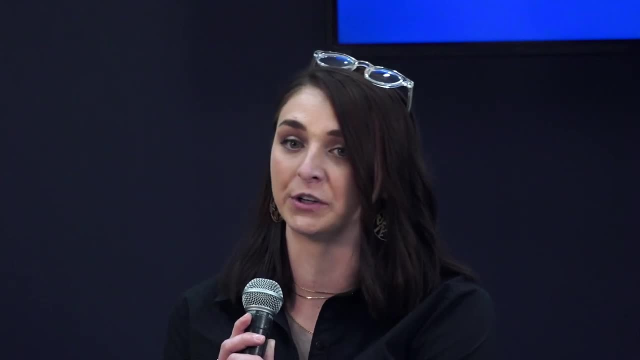 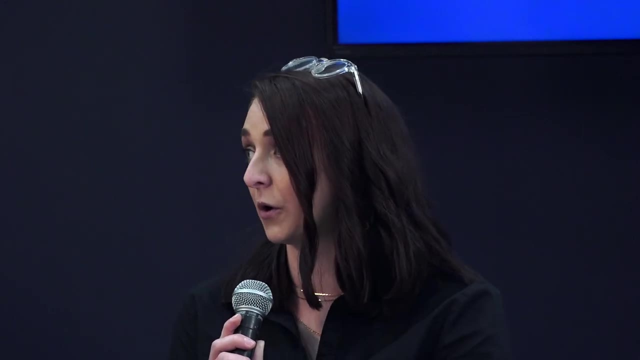 this is all about the globalization- and it's not necessarily what we would traditionally think of it, but creating those cross communities. and then from there, when we have a strong foundation between our own microbiologists, then we can take that even out of ASM and start working with other organizations. 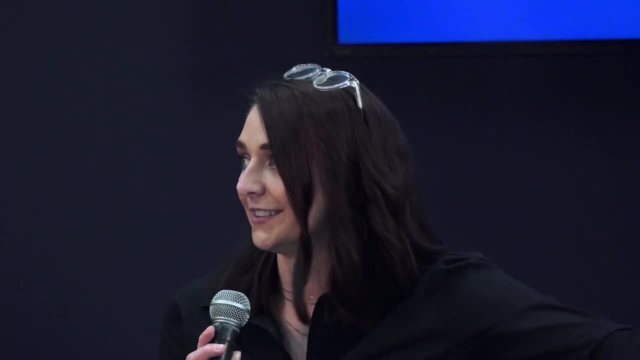 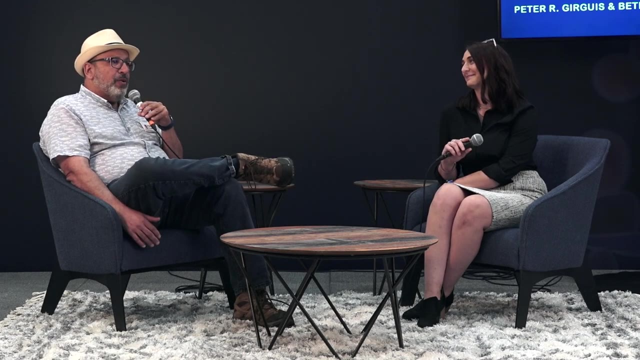 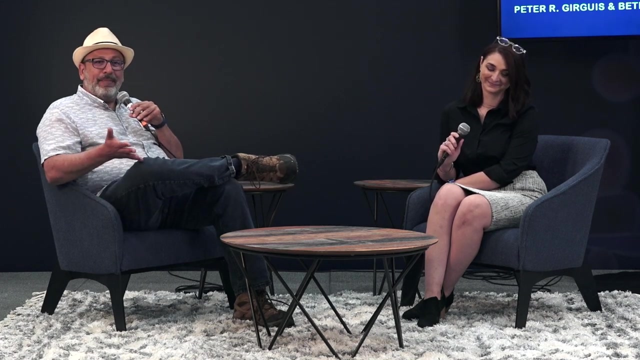 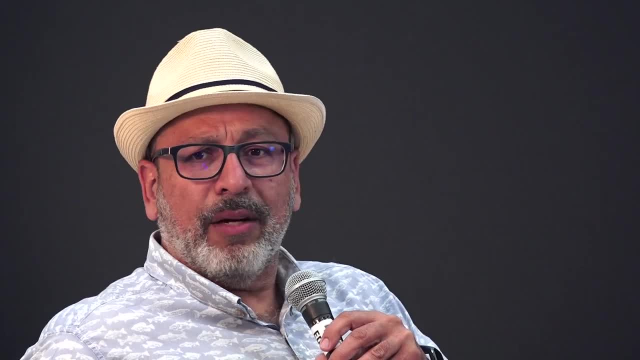 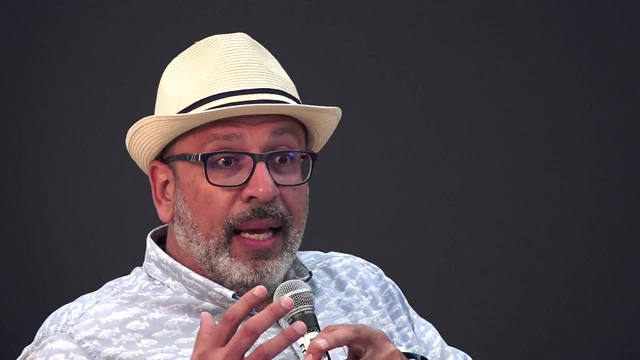 and there's a kind of culture that builds around microbiology and there's a kind of research and then the antibiotics and antibiotic resistance community, And what that tends to do is keep us to kind of rather inward looking. right, And what was? 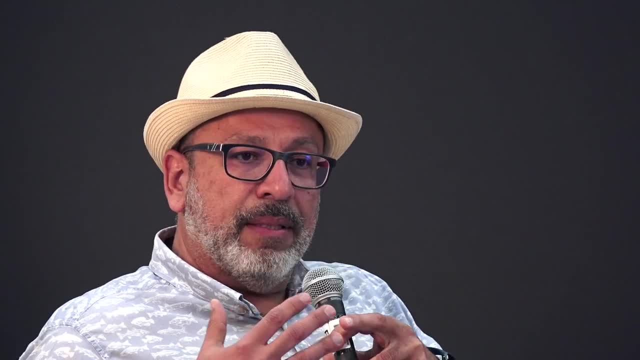 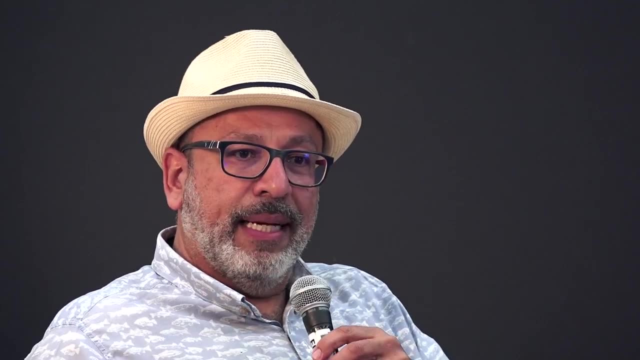 inspiring to me was to see ASM government step up and say, okay, EEB, you have something to offer, and it's this kind of perspective on how to relate different complex data sets. But in turn, other communities have a lot to offer us. So I'm an environmental microbiologist who studies. 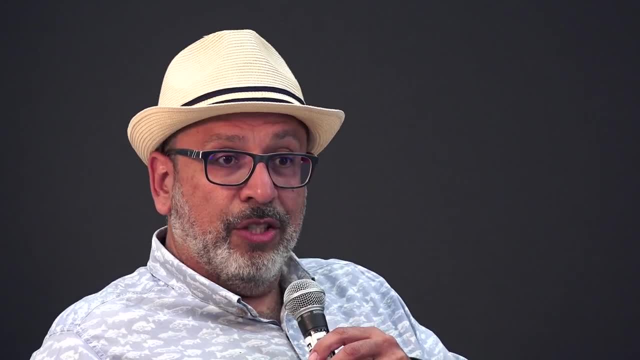 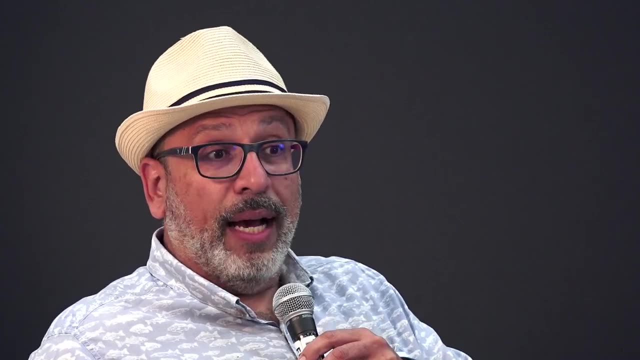 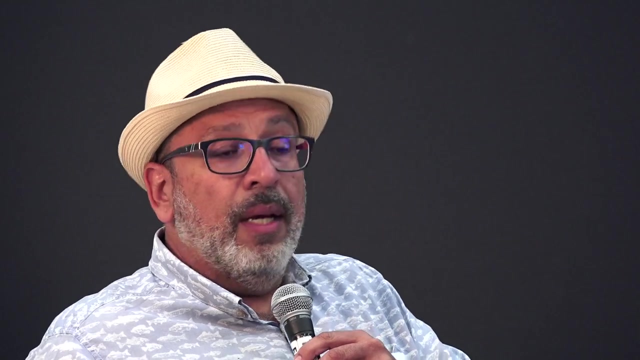 what microbes do in the ocean And understand their relationship to animals and symbiosis. I think a lot about how they shape biogeochemical cycles, even make rocks- But in many ways I don't have the kind of depth of perspective that my colleagues who study, for example, a human microbiome or livestock or other. 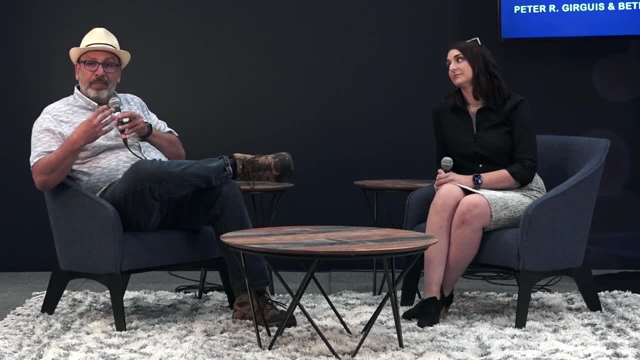 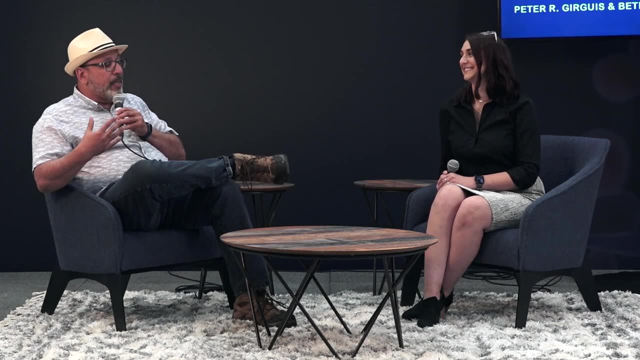 insect symbioses- right Folks that have a model system that allows them to gain deeper insights. So I see an opportunity also for EEB to learn from other communities, And you know, one of the things, Beth, we talked about was how to facilitate this kind of exchange. 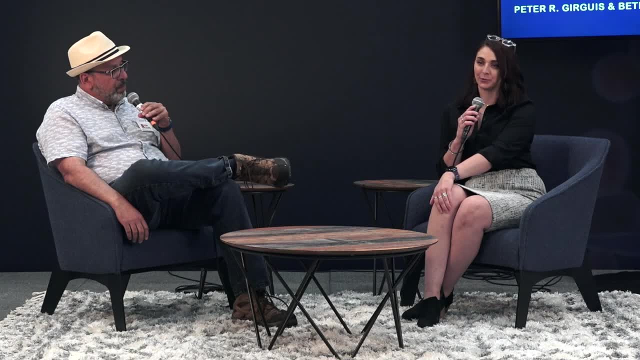 I don't know if you want to speak to that, Yeah. And again, that kind of goes back to the more we get into our own specialties- And I mean, think about when I was doing my dissertation- like that's an own language. 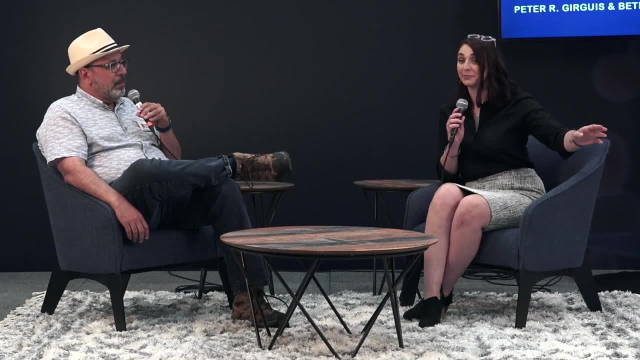 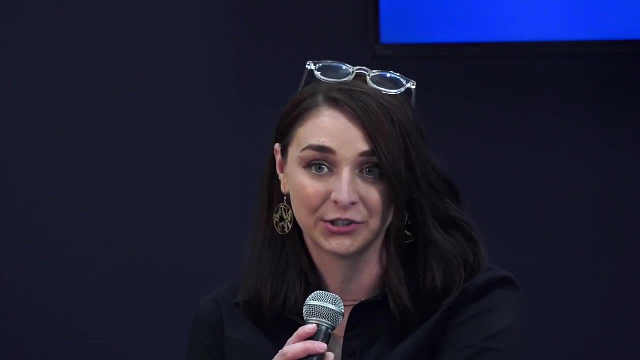 that's separate And like trying to take that out of even my own department and talk to other grad students. they're like I don't know what you are talking about, And so I think that that kind of goes back to the more we try and distill. 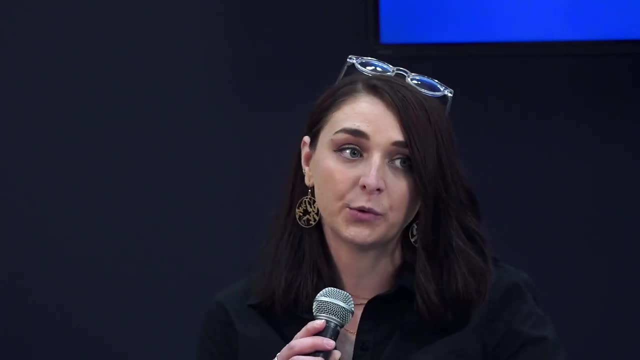 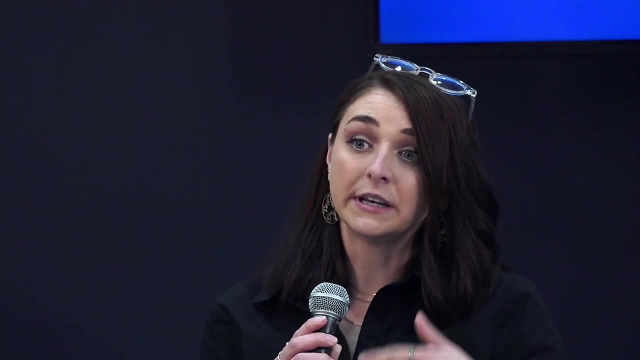 it down into these different silos, the more you end up creating an accidental new language. So then you have to take a step back and you have to be like: okay, we need to be able to communicate, And if we can't do that just between humans, then how are we supposed to? 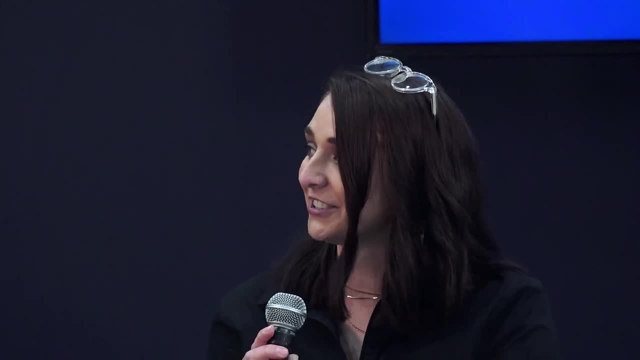 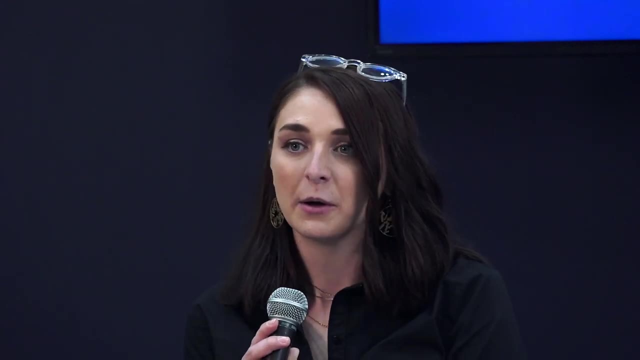 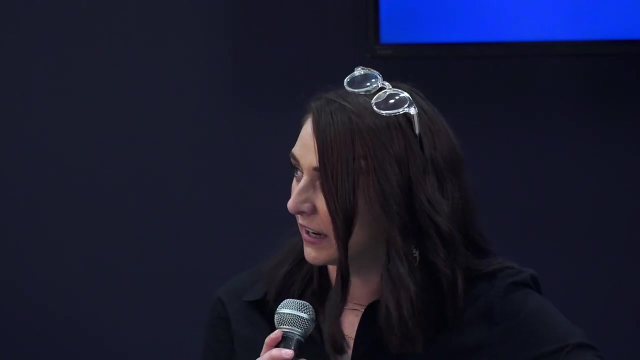 expect that to be shown across the data. And so now we have talking about these big data sets, talking about the omics, the whole bunch of different types of omics, but the way that we can utilize- Right, It might be very similar methodology, but what we end up looking and taking that data. 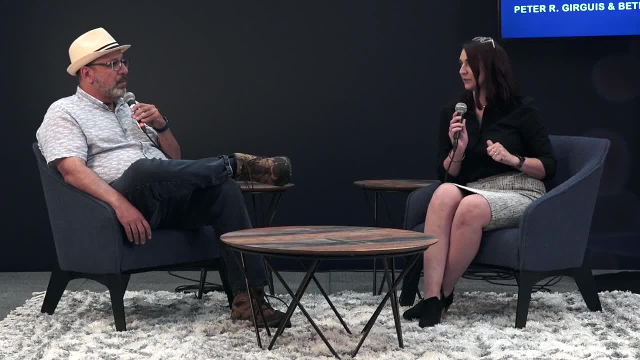 looks so different when you go, okay, yeah, we're going to do a whole bunch of mass spec and they're going to do that with the host microbe, And when they publish it it looks very different than if you did mass spec and then you took it from the ocean and that type of sample. 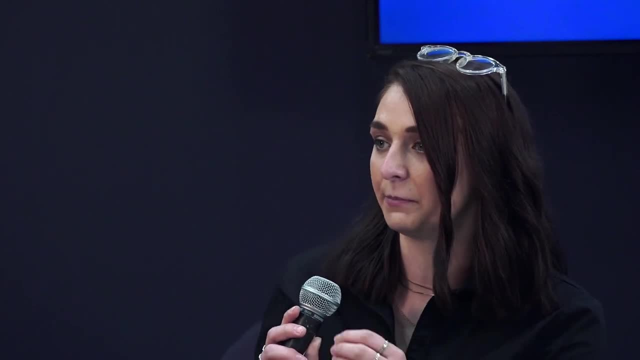 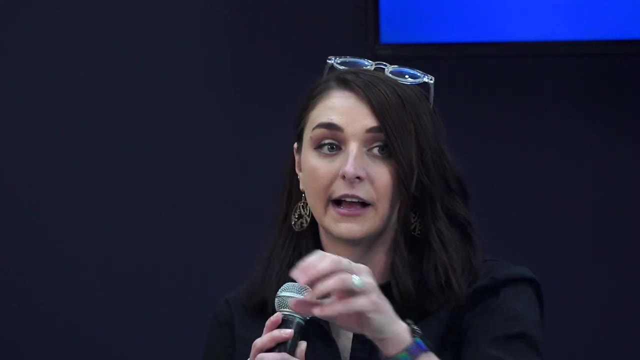 And so you have again where ASM has the ability to see where it is. We can see where the microbiologists are, what we're doing, what all of them are doing, and then how can we help facilitate that translation to the different community languages? 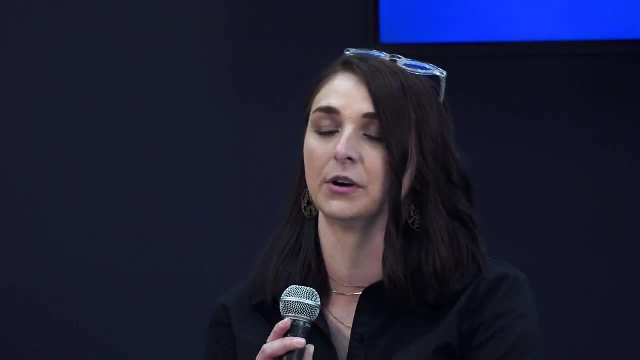 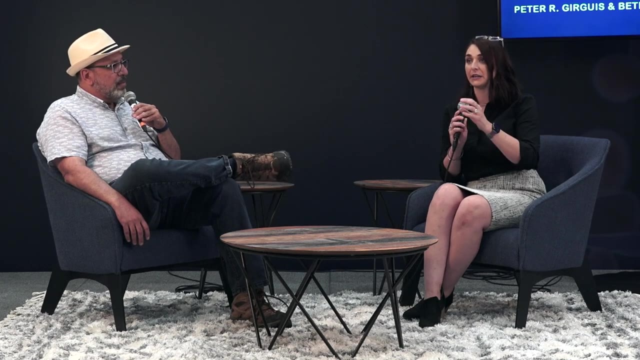 and then try and get something where we're really building on to the term hot topic of data standards, data accessibility. All of that can be done through ASM as a foundation, by working with the members who have the specialty and are excited and willing to help us then build in that translation and work across. 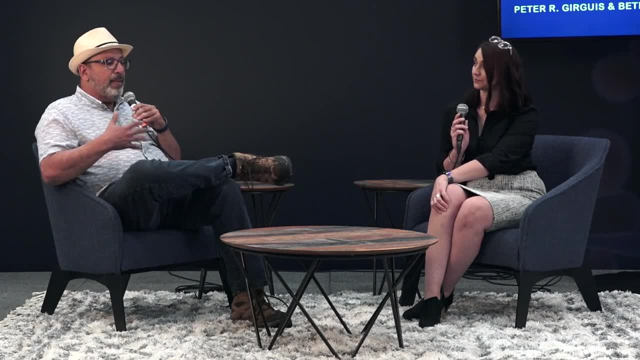 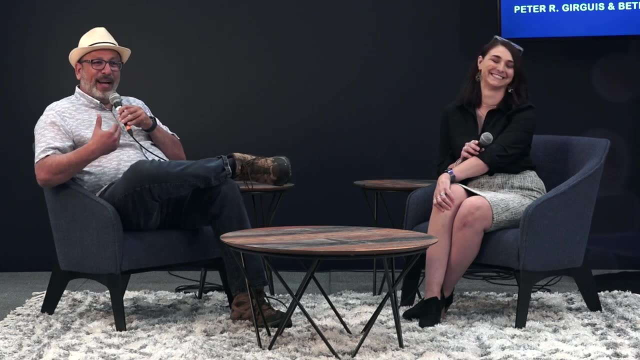 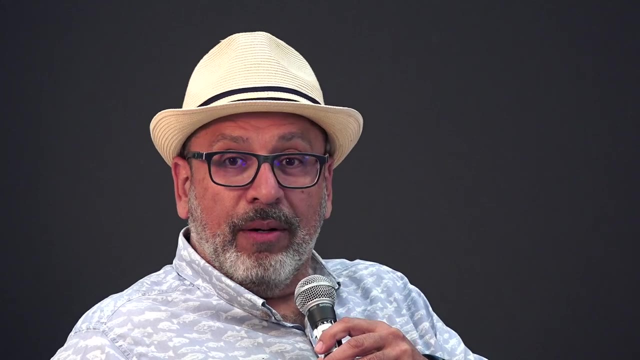 the different communities? Yeah, absolutely, And so I've been a member of ASM for about two decades, right, And let me speak with my ASM member hat on. I have plenty to do to raise the funds and to try and do my very best to mentor my early career colleagues in the lab and to try and 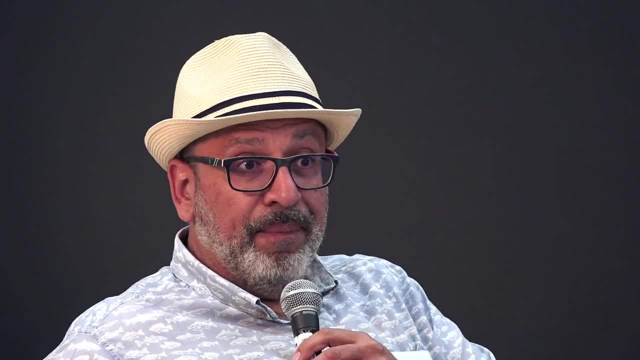 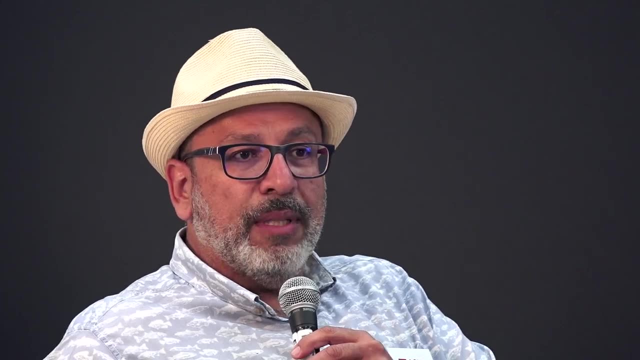 keep an eye on the advances in my discipline, And one of the things that inspires me about coming to ASM is being able to hear about others who study microbiology, And I think that's something that's very important. I'm always curious. I have a question about how we can get our microbes from a completely different vantage. 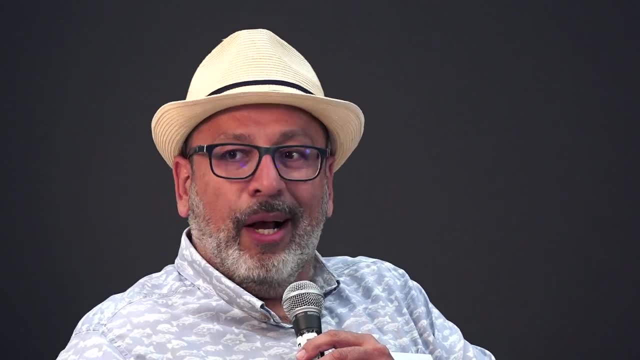 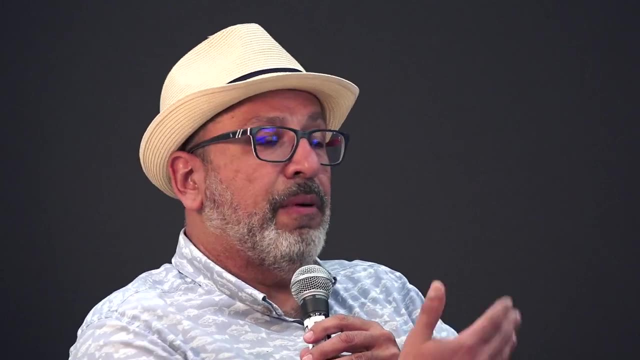 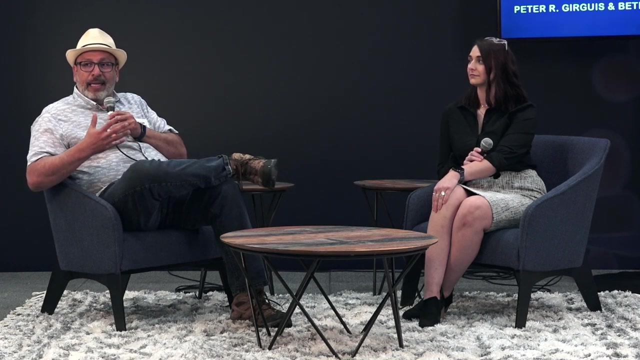 And that makes EASM a unique opportunity to really expand our understanding and thinking about how we approach our own science. And I love the enthusiasm I've heard in the voice of Beth Oates and Alan Siegel and Stefano Bertuzzi and others with whom I've worked who represent ASM governments, because I see 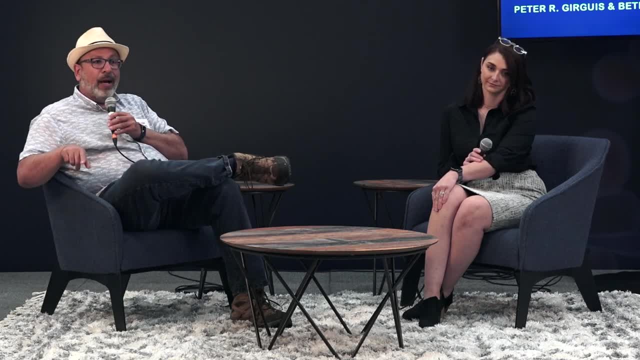 them really wanting to play a role in catalyzing our interactions. Now, I don't know how many of you all say that. I don't know how many of you all say that, But I think it's really important. I think it's really important. 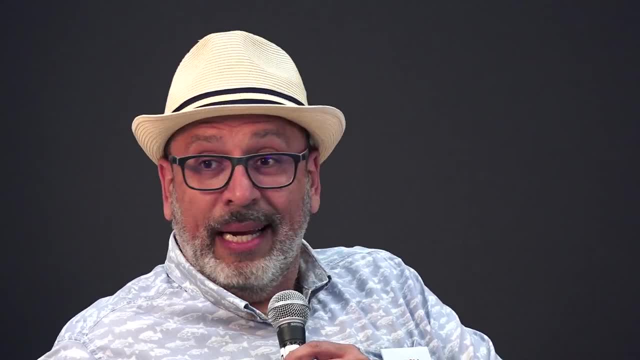 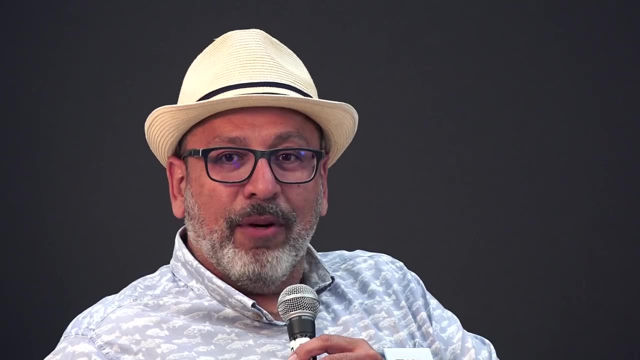 I think it's really important. sitting here joining us today are EEB. I don't know how many of you are HMB or associate with other communities, but I do know that all of us have this interest in better understanding the microbes that shape our planet and keep this biosphere alive right. So I'm really inspired by 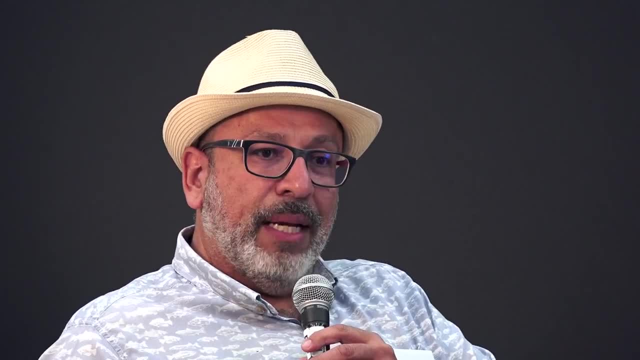 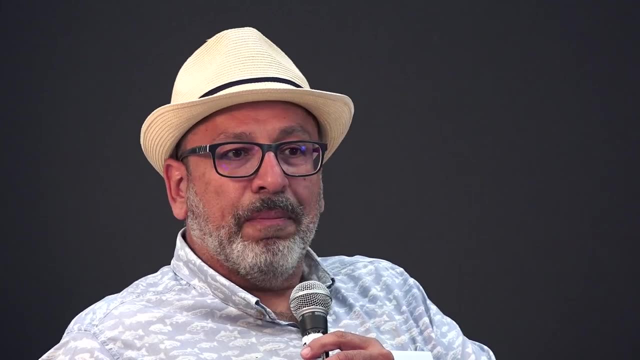 what I've heard from ASM- governance- And there's another dimension to this I want to touch upon before we turn it over to you all for your questions. ASM has an international, it's an international organization, We have international colleagues And I find that, frankly, there are. 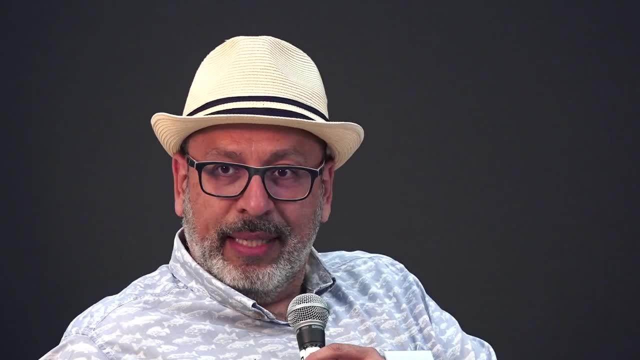 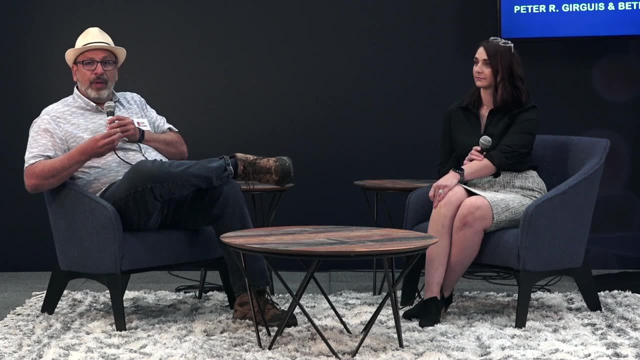 structural impediments through many US funding agencies to engaging with our international colleagues. And I think ASM is uniquely situated to really foster dialogue between those of us who are working here in the US and those working in other nations. And from my point of view, 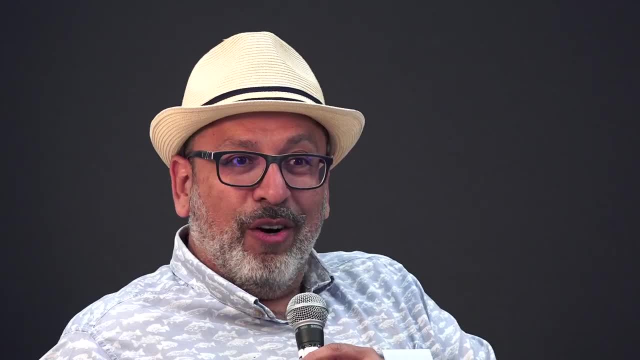 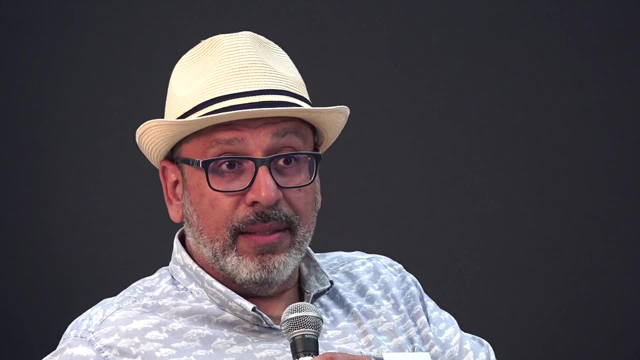 as someone who studies the ocean, the world's largest feature and arguably most complicated system, we are not going to get much farther than where we're at unless we really do truly international science, And so I'm really inspired to hear what you have to say about it. 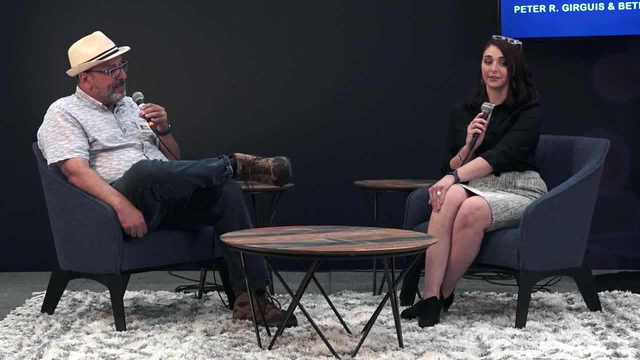 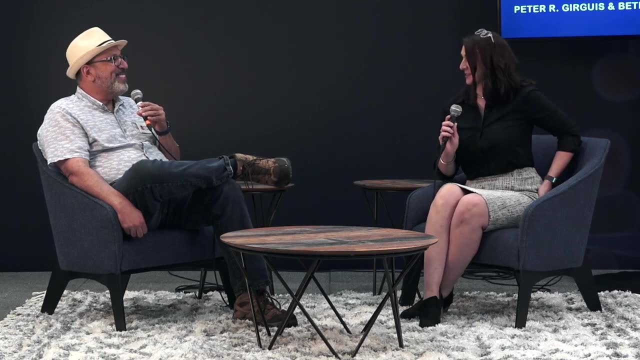 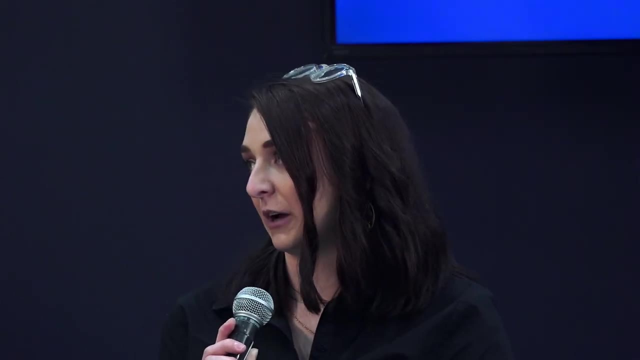 Yeah. So especially looking at ASM, we've been, although American Society for Microbiology turns out is an international organization, regardless of the American aspect of the name. But with that there's been a lot of push between. there's the Young Ambassador Program, that includes 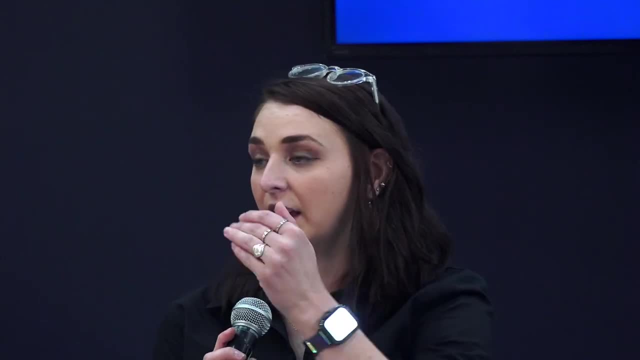 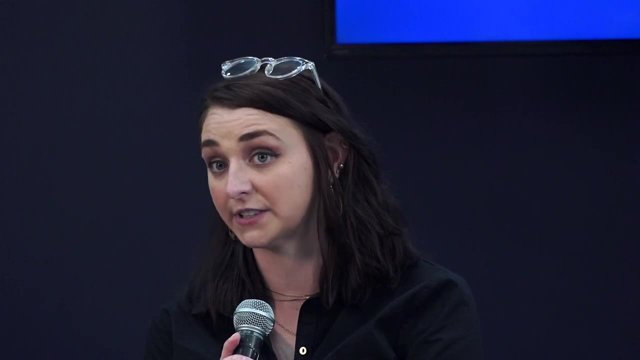 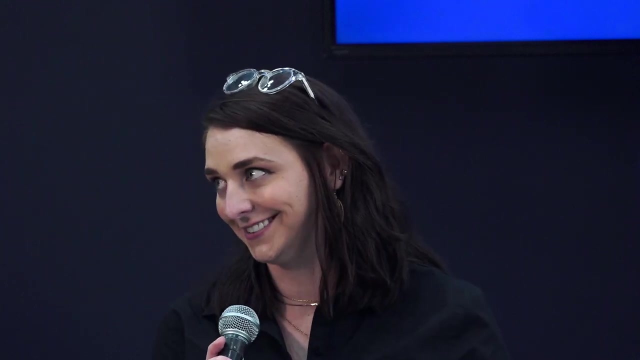 country ambassadors. There's the education And different fellowships, like trying to build into that diversity, because it's not just the diversity of its own science, It's who's doing the science And goes back to. we have the globalization. These microbes are everywhere, everywhere. So big shock our microbiologists. 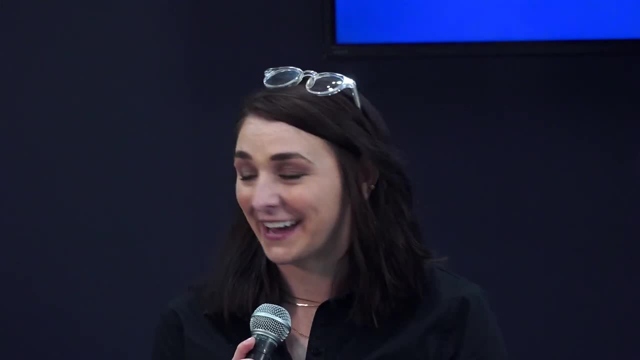 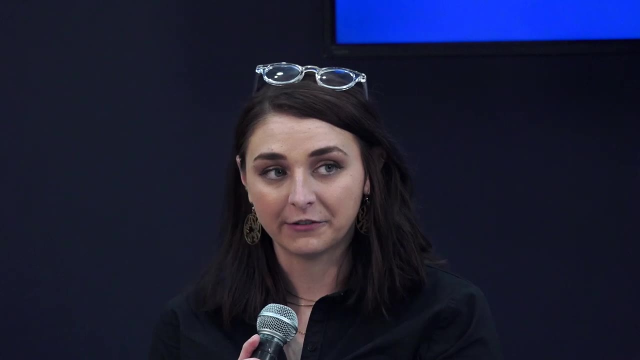 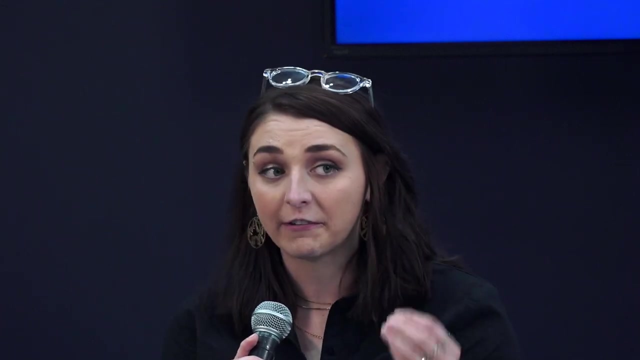 are everywhere, So kind of building that back in. that's part of the thing, And so, ASM being this big organization, the whole point is really for us to work with our members to help facilitate the conversations, to create productive changes that are effective and will. 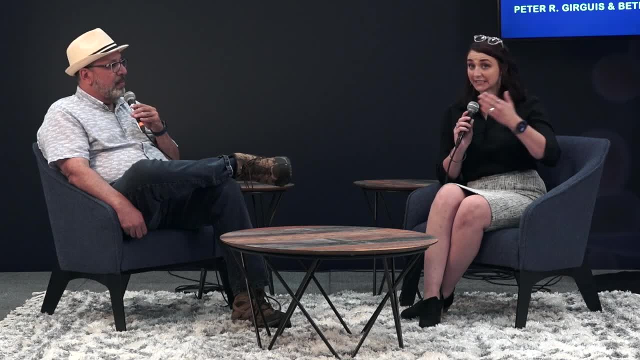 continue to push both microbiology but just science in general forward. We're at the cutting edge. We're going to continue doing the science, We're going to continue keeping it going. But it's really working with the staff and the members and trying to find those common grounds and 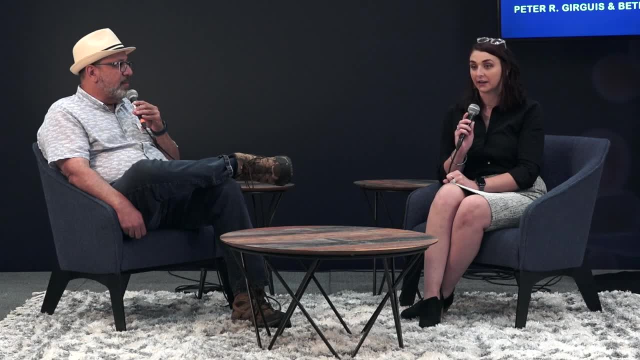 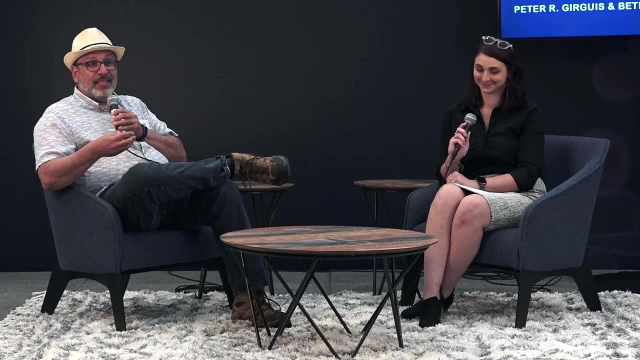 identify where's the best opportunities for us to make effective changes. Absolutely, And that was one of the most inspiring things about our retreat- was an emphasis on actionable items. Now, I don't know, Beth, if there's anything else you'd like to share before. 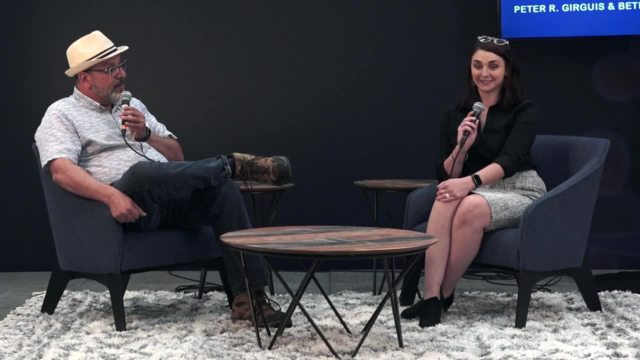 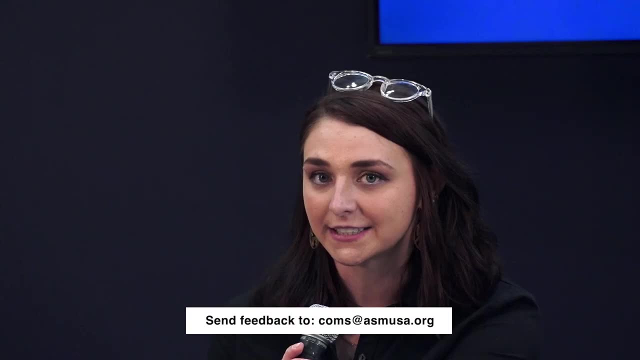 we wrap it up and turn it over. What do you think? No, I think that that's we're right at time, But I wanted to thank everybody And, if you're interested in learning more about the Council of Microbial Sciences and how we look to the 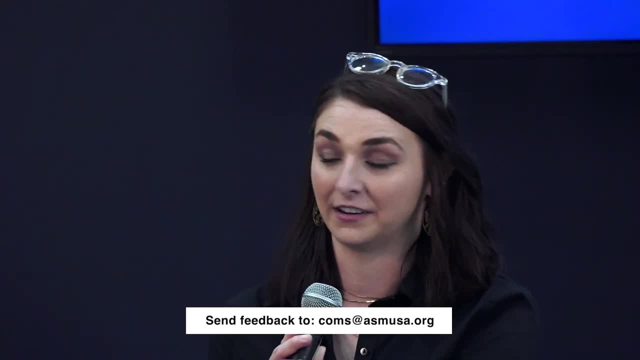 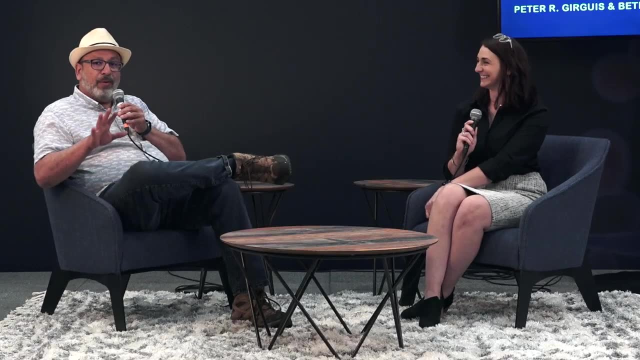 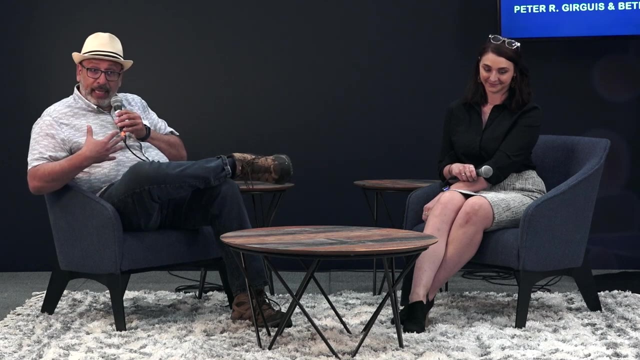 future and see where we're going and how best ASM can build us there. we're more than happy to talk to you off stage, away from a microphone. Absolutely, I have a request of you. all right, It is important that ASM representatives community.